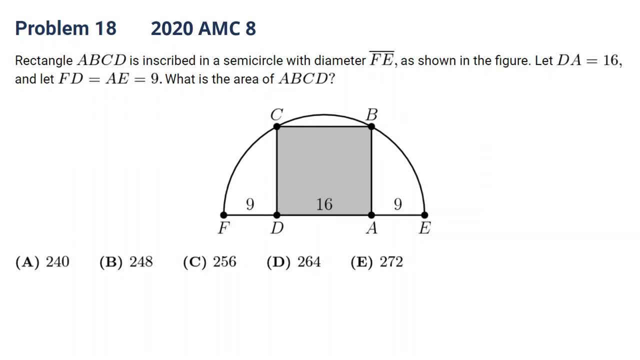 and you can see it's symmetric: 9 and 9.. What's the area of ABCD? So basically, we are looking for? if we can know this side, we are done. How can we get this side? Think about it. It's symmetric, so probably. 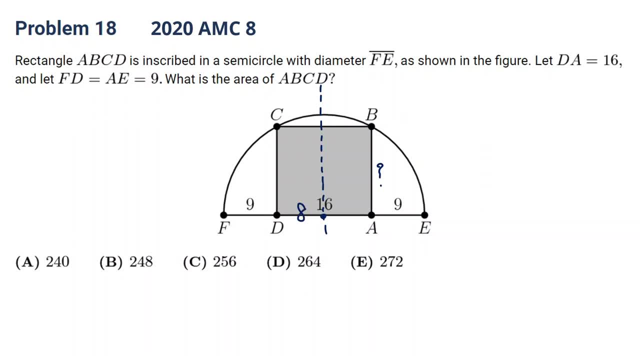 we can find the center of it. This is 8.. This is 8.. And all of a sudden we know that the radiance of this circle is going to be 8 plus 9, 17.. So how can we get the H here? We should add a line. This will be the same as the radiance. 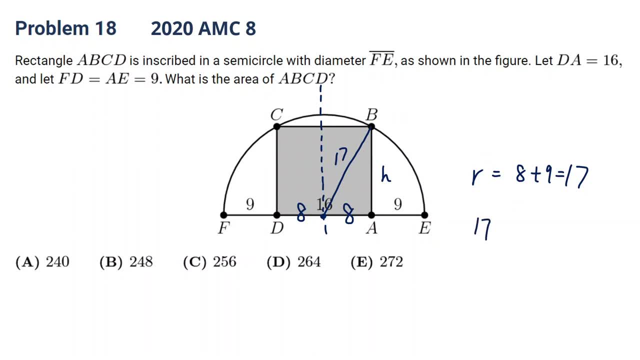 17.. Okay, now we can get the height. It's 17 square minus 8 square square root. This is so today I want to introduce another algebra trick. So you know, A square minus B square is the same as. 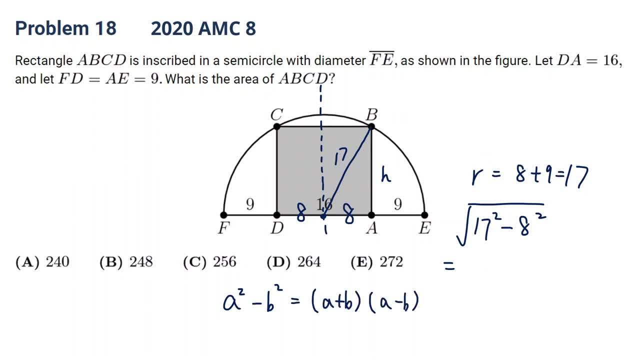 A plus B times A minus B. So, for example, 5 square minus 4 square will be the same as 5 plus 4 times 5 minus 4.. This will be very, very helpful in our calculating if you are not allowed to use a. 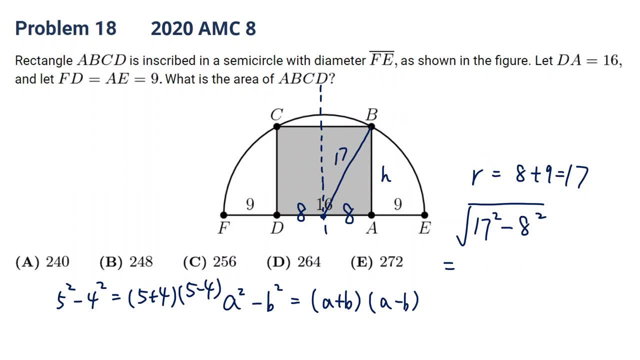 calculator. This is like a calculating trick. So here, 17 square minus 8 square is going to be 17 plus 8 times 17 minus 8 is 25 times 9.. That is 225 square root. This will be 15.. So now we get: the height is 15,. 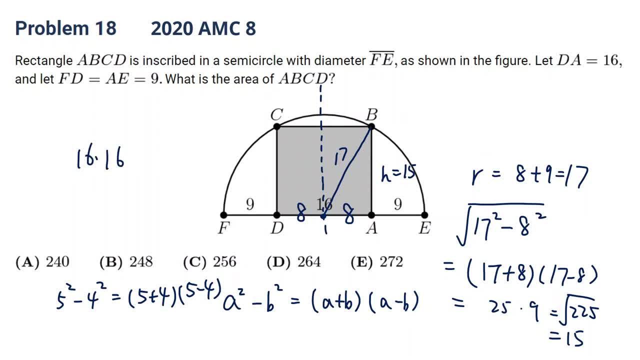 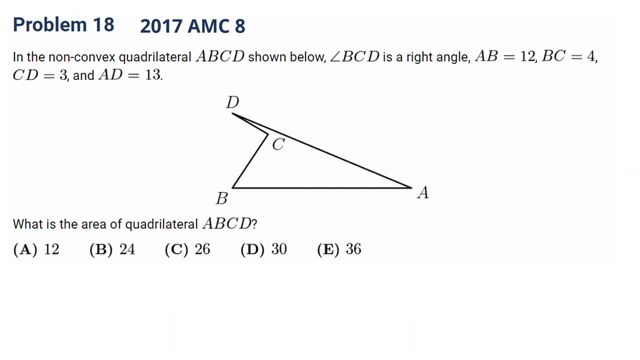 so the area will be 16 times 15, that is, 80, 240,. okay, Like I said, it's not not as straightforward. You sometimes, in Part B questions you need to add one line by yourself. Okay, let's see another one. This is 2017, problem 18.. Let's.